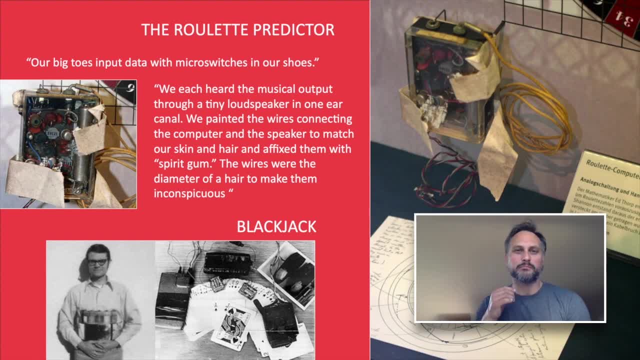 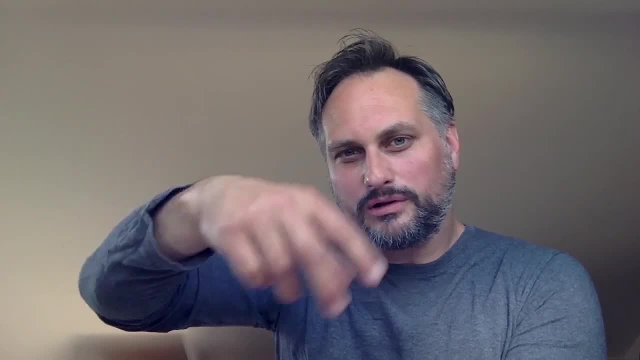 with your big toes and the output would be mapped to a tiny loudspeaker in the form of music playing to you. Depending on when the copier would have set off the ball, you flipped the switch: The last tones. counting down the last tones stopped would indicate which opt-in you need. 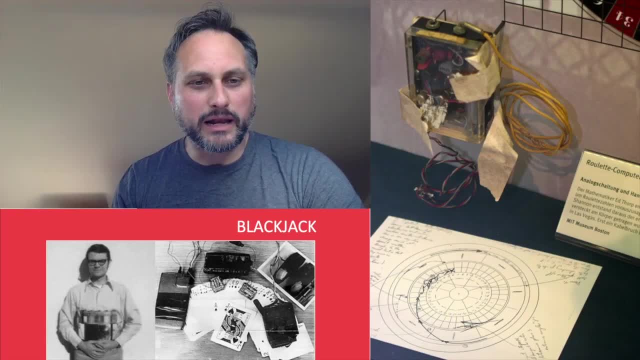 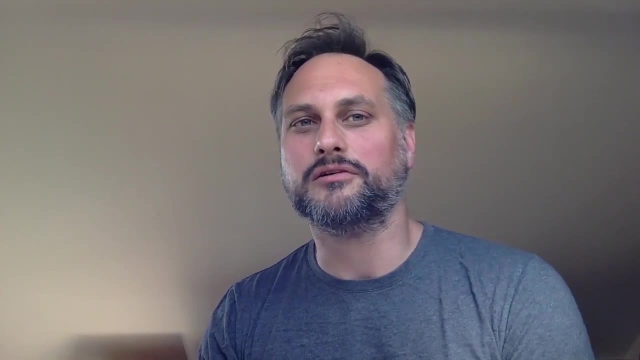 to bet on. Thorpe also built a blackjack prediction machine, which you can see below just as a side warning, both of which he quite likely would get into big trouble if you would ever try to wear them into a casino. Nonetheless, important milestones in the history of computing. 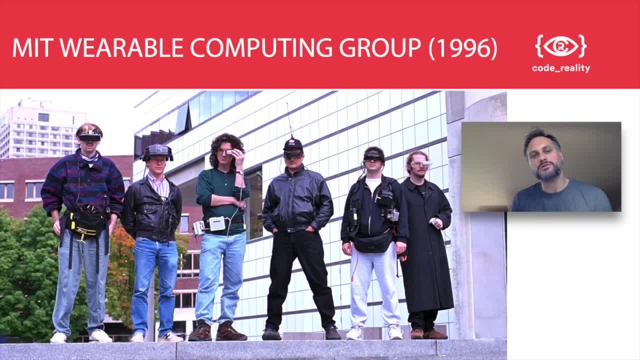 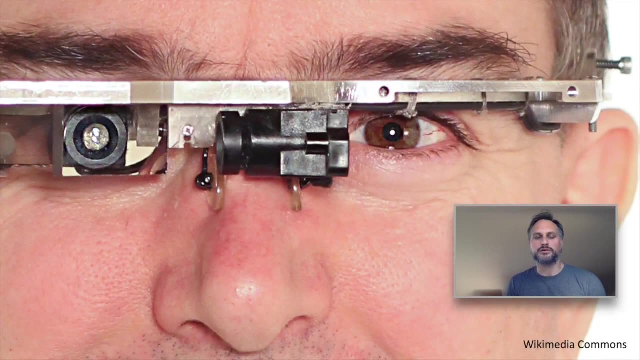 A similarly important milestone is the invention of the first generator. The first generator was the general-purpose wearable computer by Steve Mann, who you see on the left here from the famous group photo of the MIT wearable computing group in 1996.. Steve Mann built various forms of smart glasses here, a prototype fourth generation that would 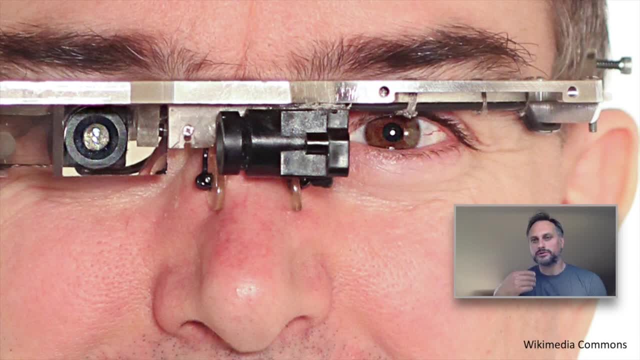 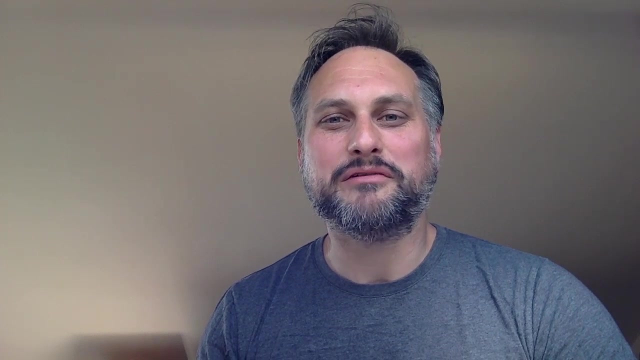 be attached to his skull. that allows users on the internet to follow what he is seeing and to text him messages directly to his eyes so he can read them from it. A couple of publicity stunts may be available- very interesting stories to read about how. 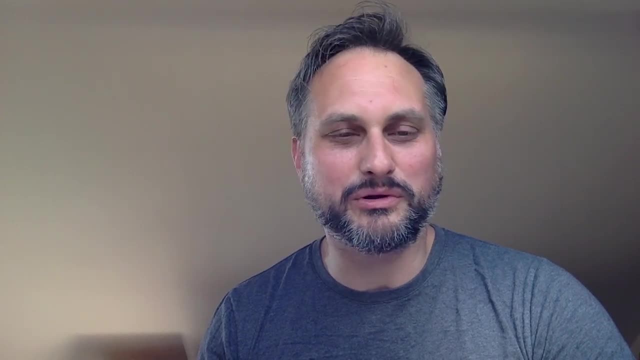 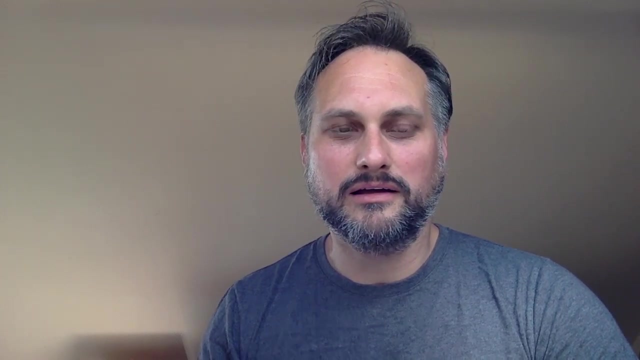 Steve Mann was harassed by McDonald's staff wearing that wearable computer and so on and so on. It's definitely worth a look and it's definitely a milestone in the history of computing. In Steve Mann's definition, in the old definition, a wearable computer is a data processing system. 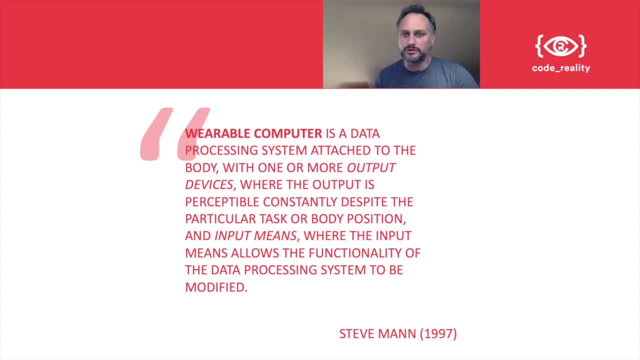 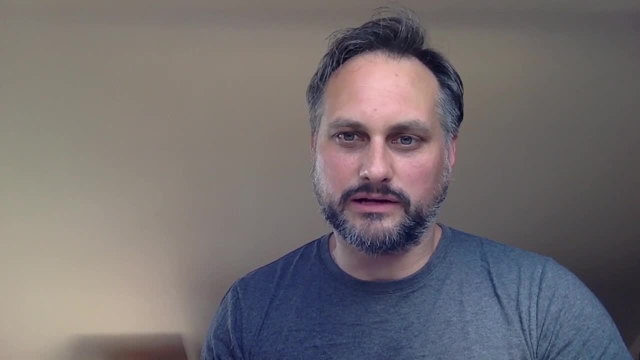 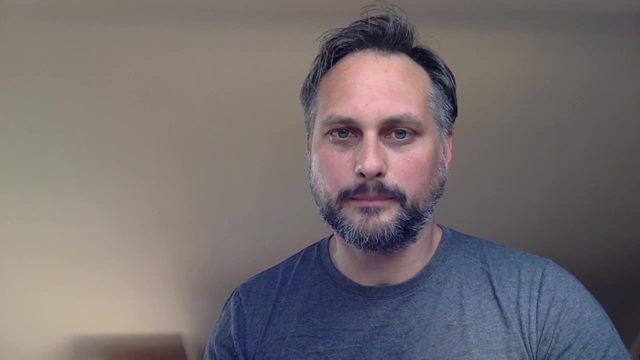 that's attached to the body with one or more output devices. Output is visible constantly, No matter what you do or what position you are with input means, where the input means can drive the functionality of the data processing system. So is that where we're computing the new fashion? 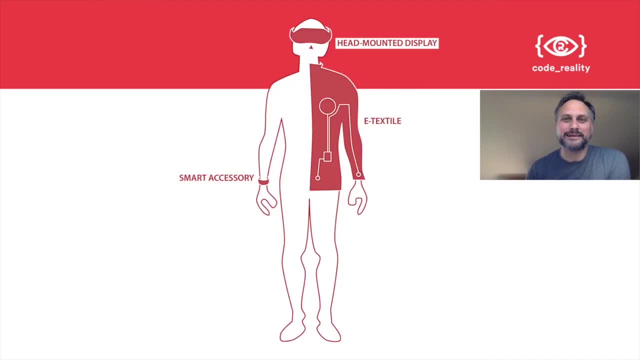 No, it's a sin, one could say. It is certainly, today, a bit different, and from this revolutionary work that we've seen, the field has certainly moved on a lot. Yeah, The field has moved on a lot towards consumer products, and that then involves also, of course, 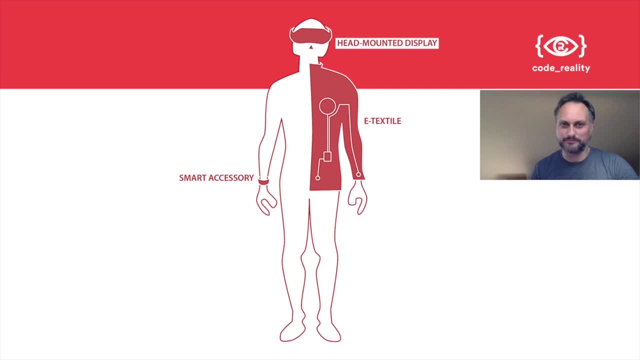 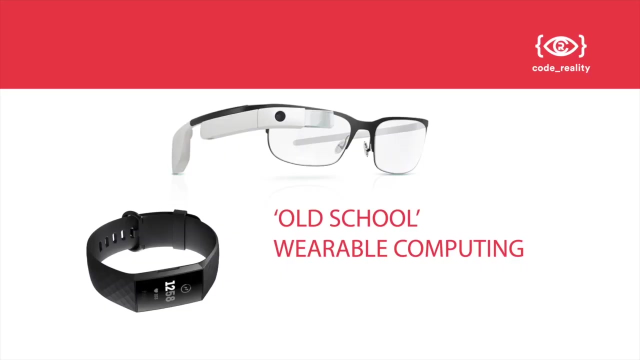 fashionable design and not just the technology. Wearable computing today falls into three classes. You would find smart accessories, head mounted displays and e-textiles, or also called smart textiles. Old school wearable computing is this: You would find accessories that you wear that have a defined design. 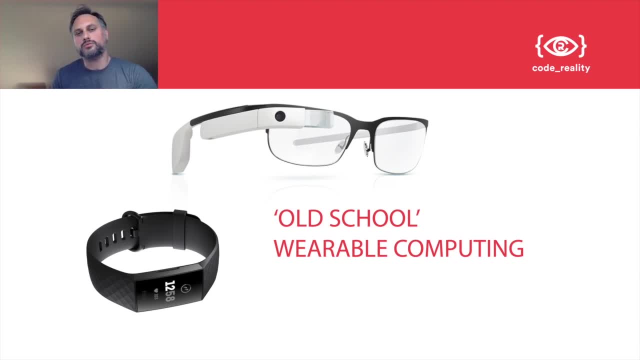 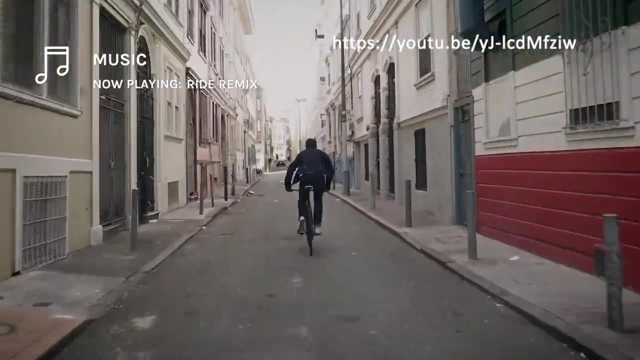 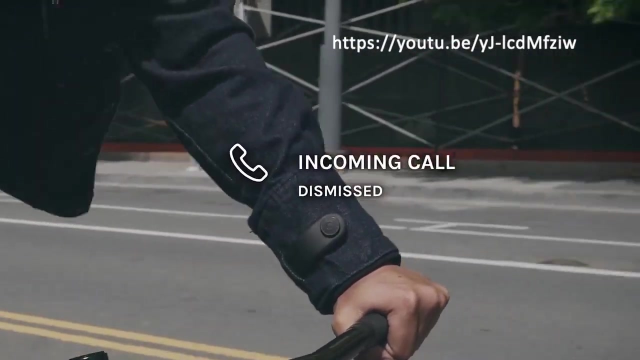 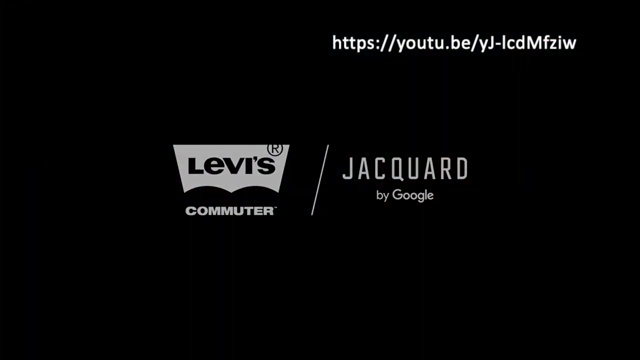 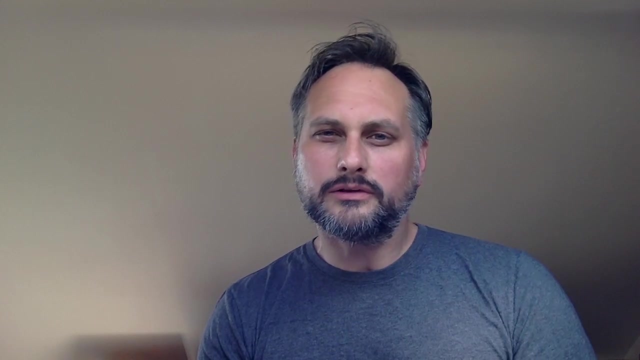 find designed form factor. you react to things in the environment, possibly read values from a display that is integrated in one form or the other, but the field has changed and today things like this are possible. so what is the theney school of smart textiles? smart textiles are able to. 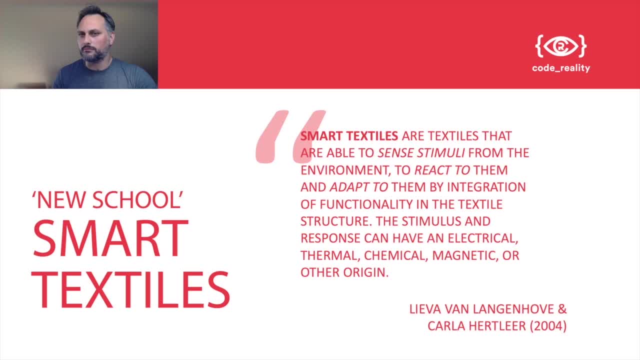 send stimuli from the environment, react to them and adapt to them by integration of functionality. 딱 하는品이라고니 에� job, one of the example in which didn't look 곯igung tool or smart textiles. smart textiles are able to send stimuli from the environment, to react to them and adapt to them by integration of functionality. 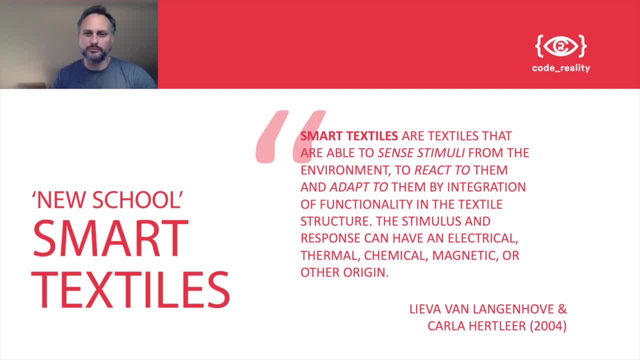 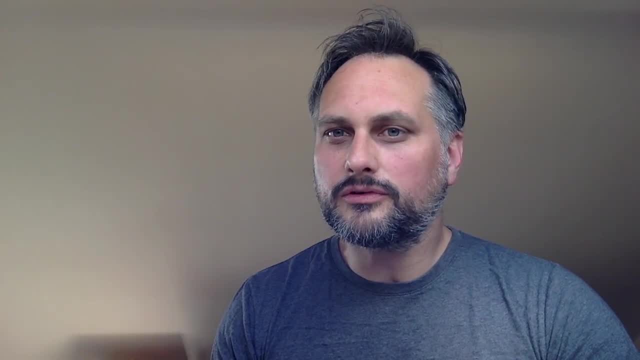 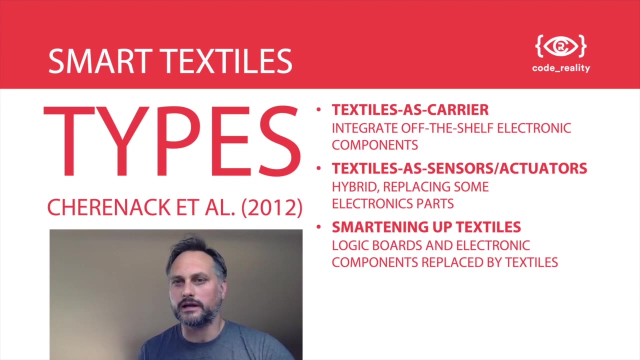 directly into the textile structure and that can have many forms: electrical, thermal, chemical, magnetic or of other origin. Smart textiles again fall into three different types of classes. if we look at the way they are produced, We find textiles as a carrier, where the textile is just integrating off-the-shelf electronic. 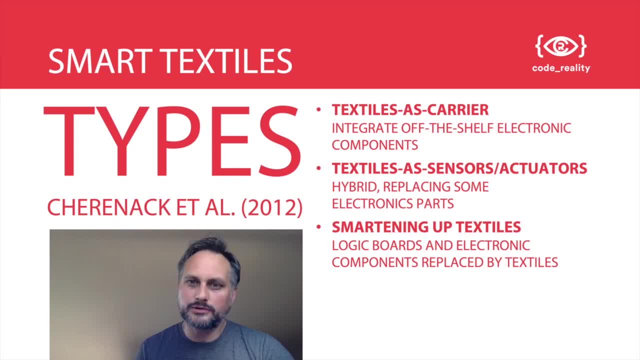 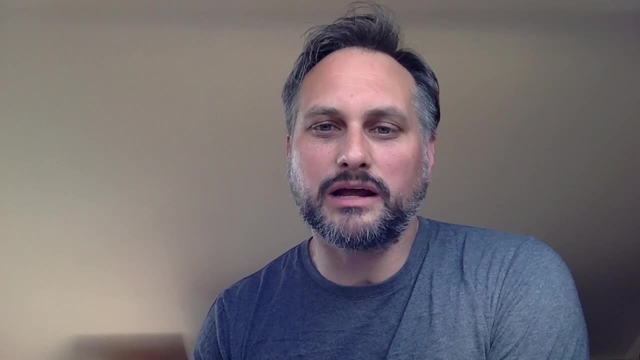 components. Then we have textiles as senders or actuators, which are hybrids, so they replace some of the electronic parts, but quite typically they would come with a main board integrated and just a sender or an actuator. But there is also the possibility to smarten up textiles completely and replace any of 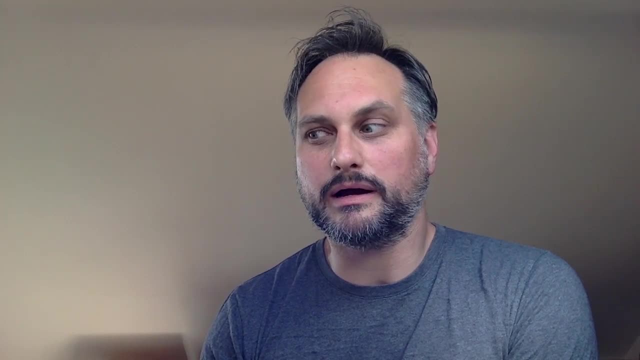 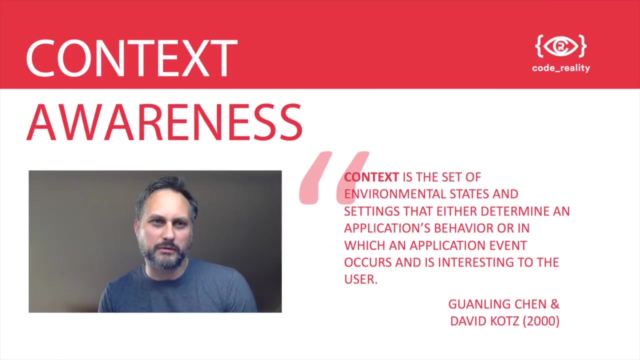 the logic boards or electronic components by their equivalent built from textiles. What is significant to all smart textiles is their ability to provide context awareness. Context awareness is the ability to provide context awareness. What is a? the set of environmental states or settings that determine the behavior or 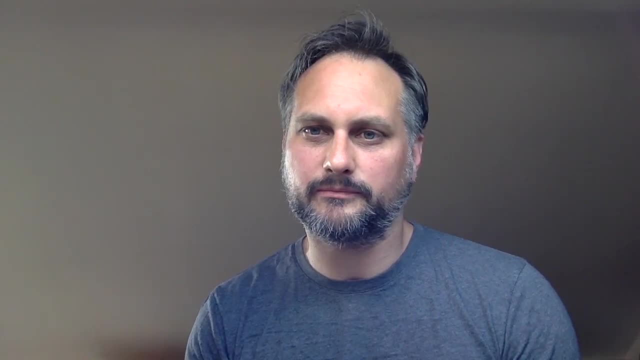 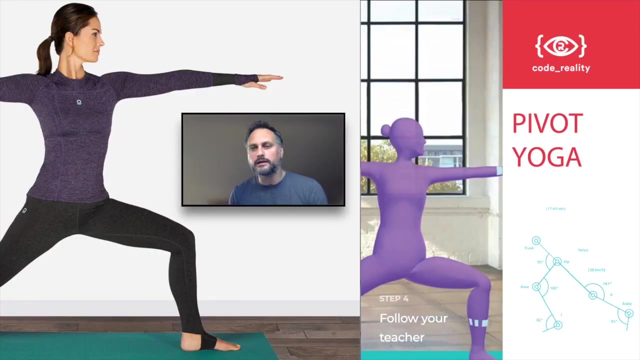 an application event that occurs and is interesting to the user. An example we find here is Pivot Yoga'sற yoga dress with integrated sensor that allow the application to monitor how the user is moving and provide feedback on that within the limits of what you see as textiles. 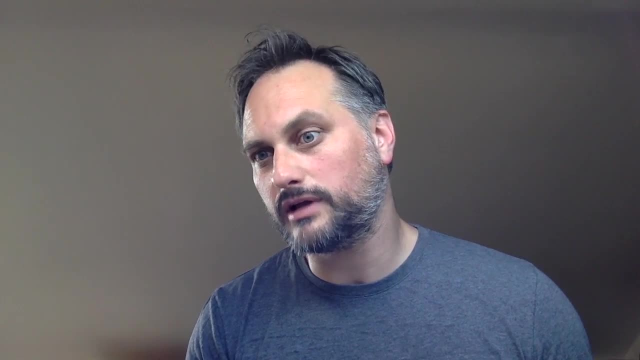 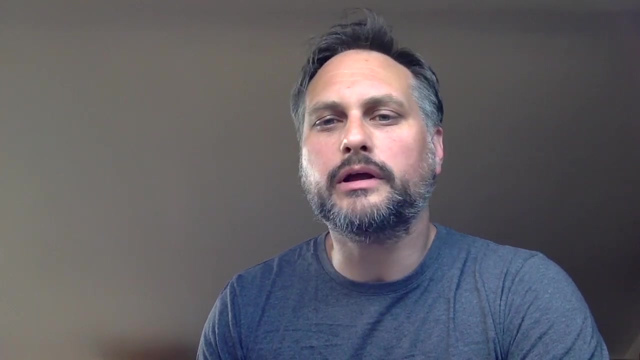 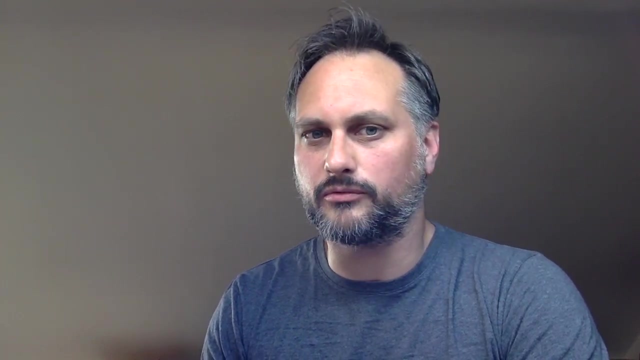 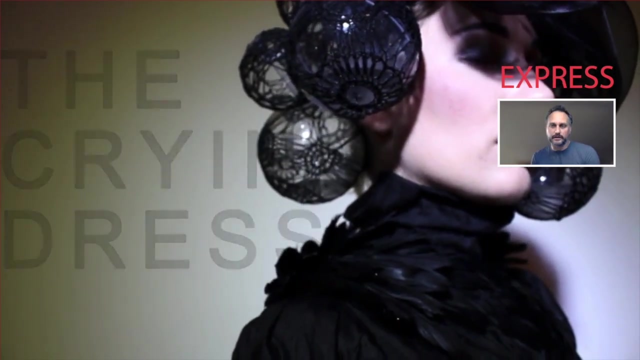 you see on the right of the angles sensed by the sensors. Why do we wear? We wear to express, communicate and protect, And I brought three good examples to underline how that actually works. The first one here is Express. This is Coca Buns crying dress, which has integrated actuators to 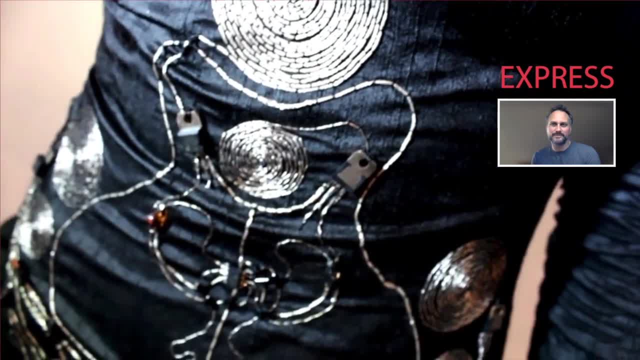 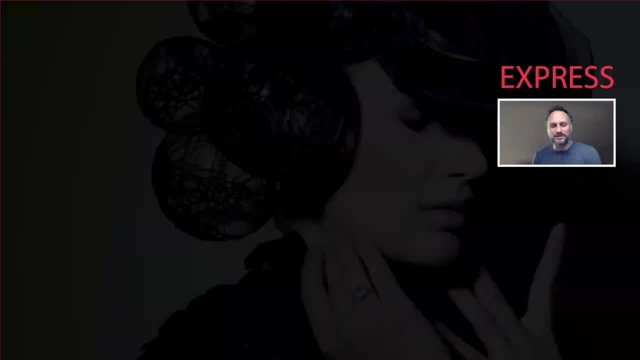 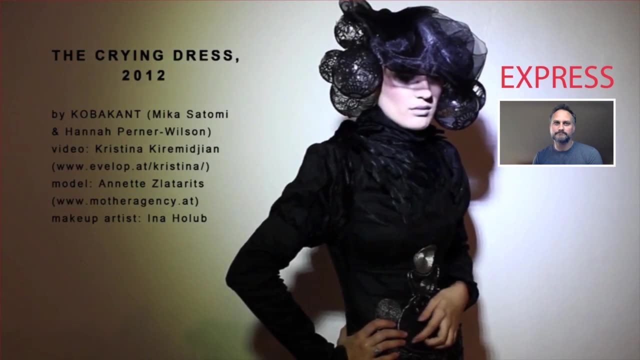 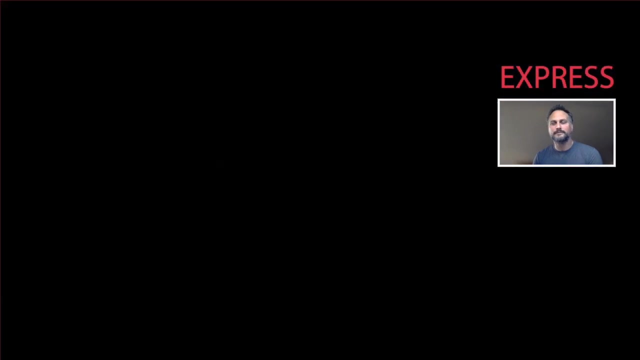 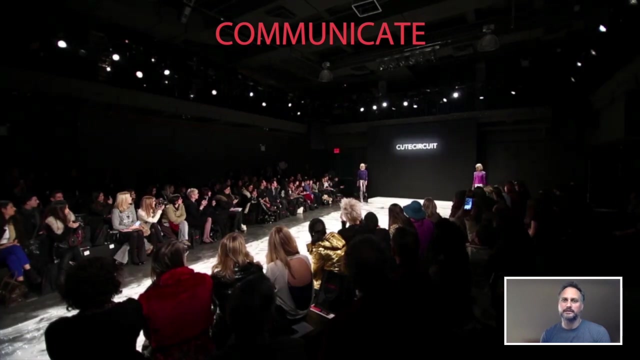 produce tears. This allows us to express emotion. This is certainly a very haute couture example, but you can see what's what's possible with wearable computing. The second example is a t-shirt that communicates with the environment. It communicates a sensing t-shirt from cute circuits. 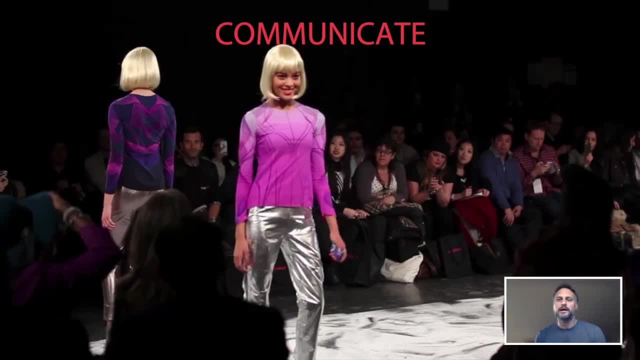 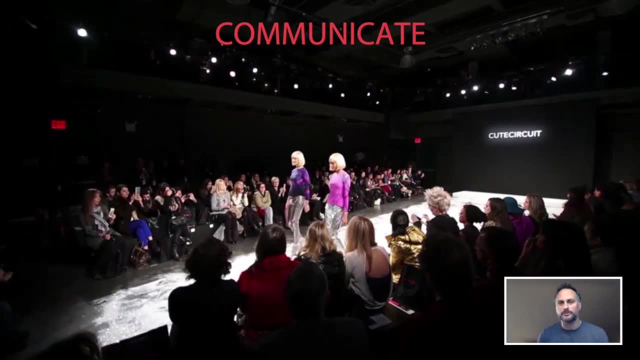 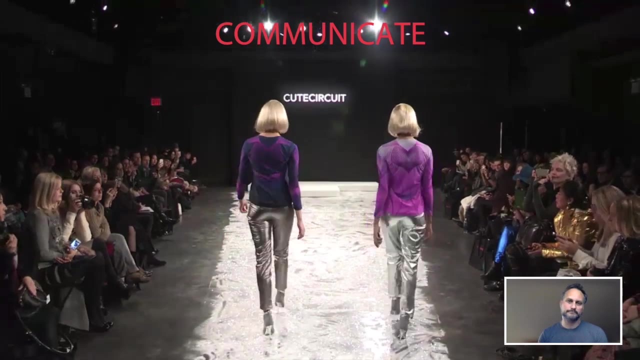 The two t-shirts are linked up and touch provided to one of the t-shirts is linked to the other, so they wear a feeling to the hug. The second example is a t-shirt that communicates with the environment. The second example is a t-shirt that communicates with the environment. 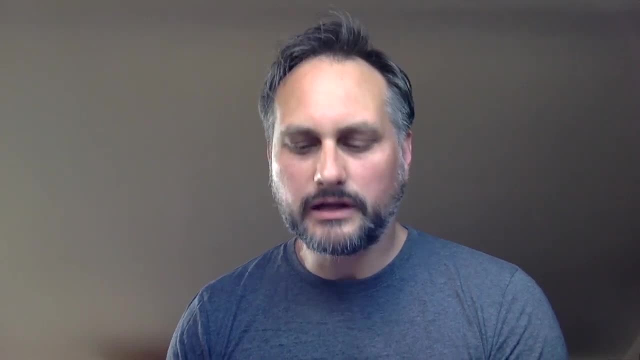 The third example is a t-shirt that communicates with the environment. The second example is a t-shirt that communicates with the environment. The third example is a t-shirt that communicates with the environment. So that's what we wear to communicate. The third example is protect.